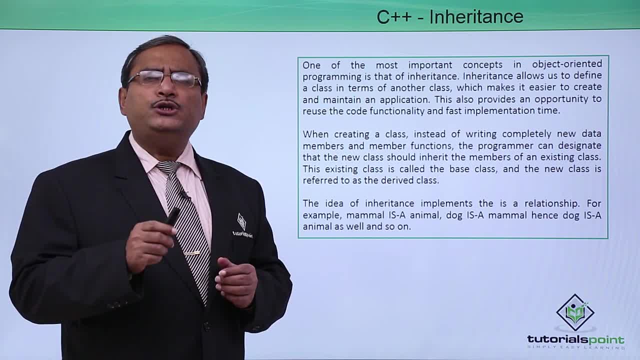 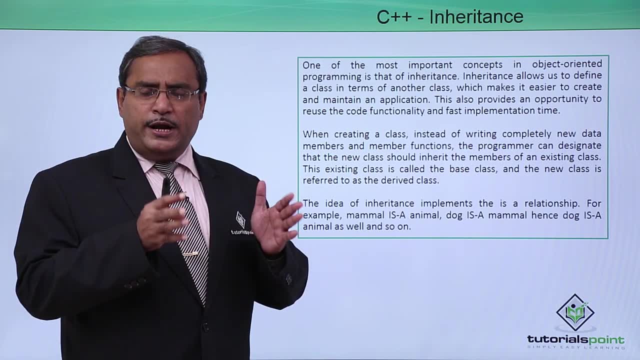 Whenever you are trying to write one class, why should always write the class from the scratch? If you find that there is one class where the codes are pre-written which are required in another class, then we shall go for the inheritance And inheritance. 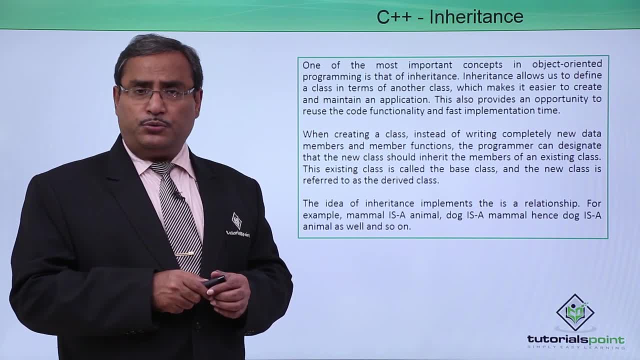 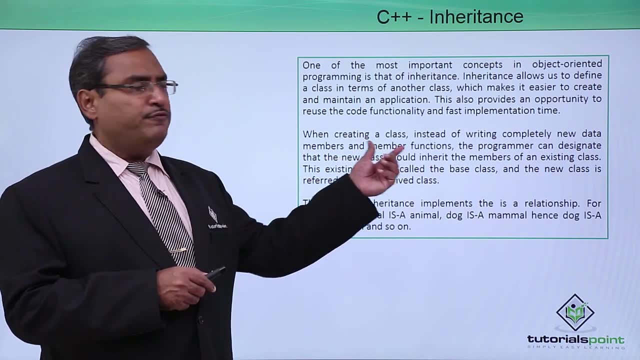 is one of the very important features in object-oriented programming. When creating a class, instead of writing completely new data members and new functions, the programmer can write a class from the object-oriented programming. The programmer can designate that the new class should inherit the members of an existing class. 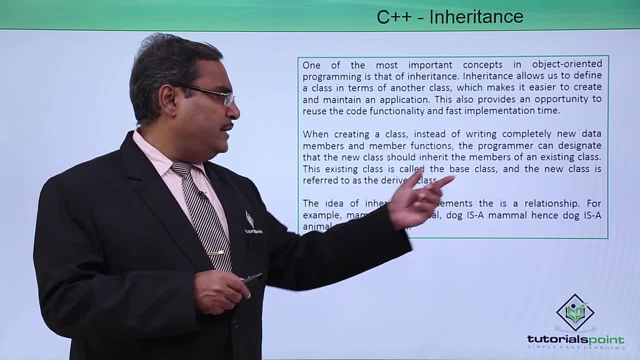 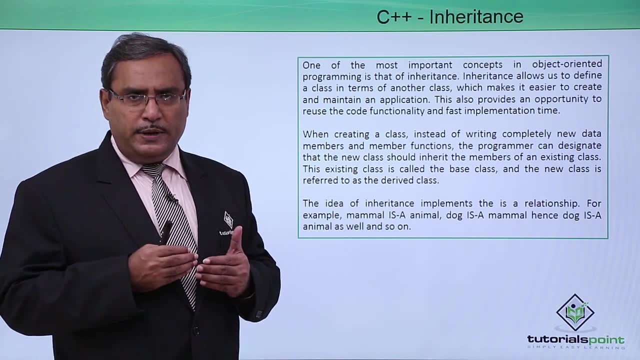 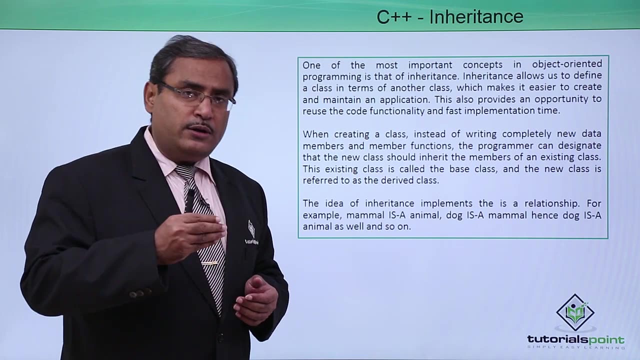 and the existing classes will be called as the base class and the new class which is referred to be will be known as the derived classes. So from a class, another class will be derived, So the class which will be obtained ultimately will be known as the derived class. and from where will? 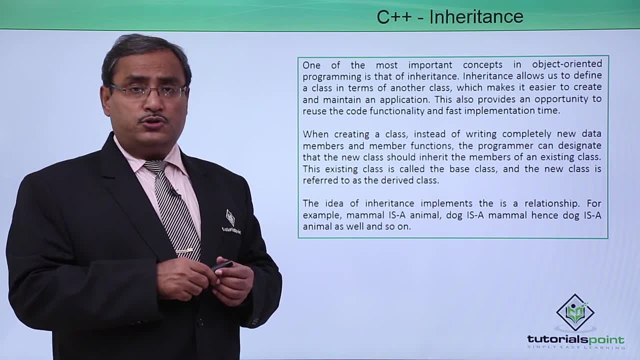 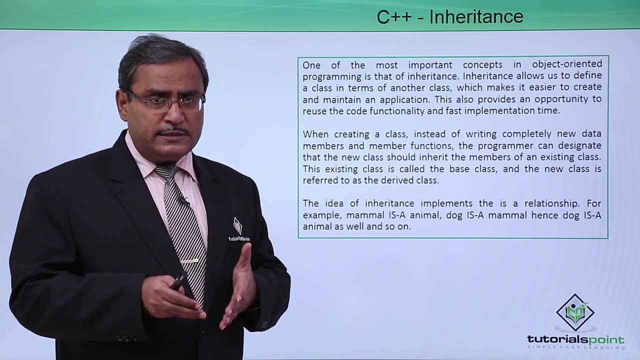 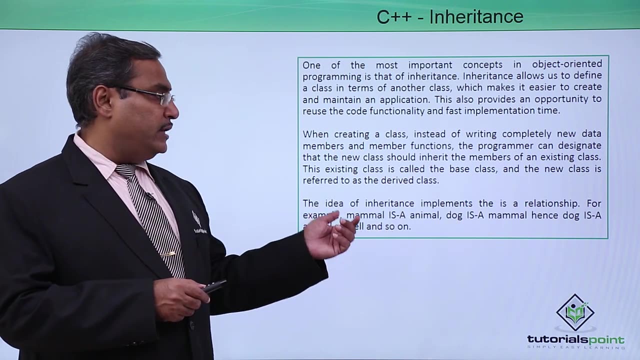 be taking. the properties will be known as the base class. So a base class can have multiple derived classes, and converse is also true in c plus plus that means a derived class can have multiple base classes. The idea of inheritance implements: the Is a relationship. for example, mammal Is a. 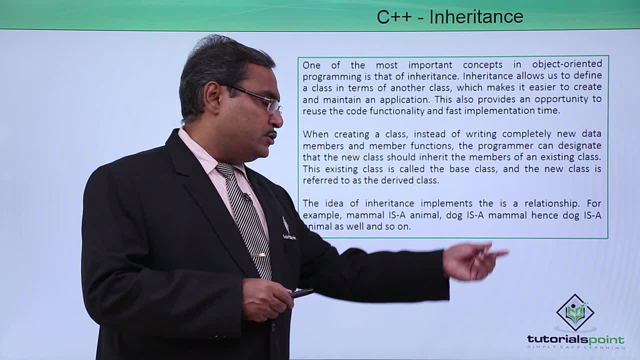 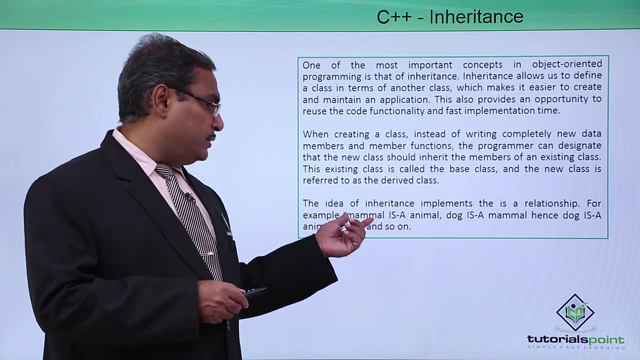 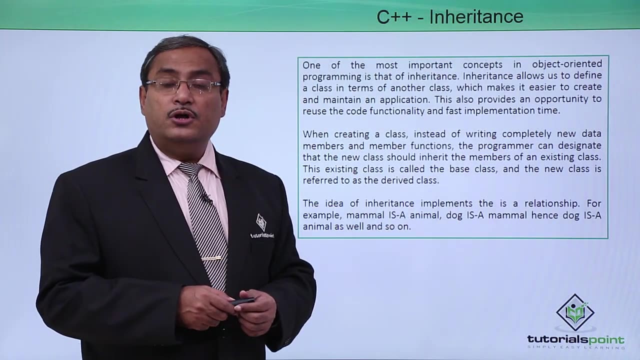 animal. dog Is a mammal, So hence dog Is a mammal and dog Is a animal as well as then so on. So here you can find that this mammal Is the base class and this animal is the derived class. So in this way the codes written in one. 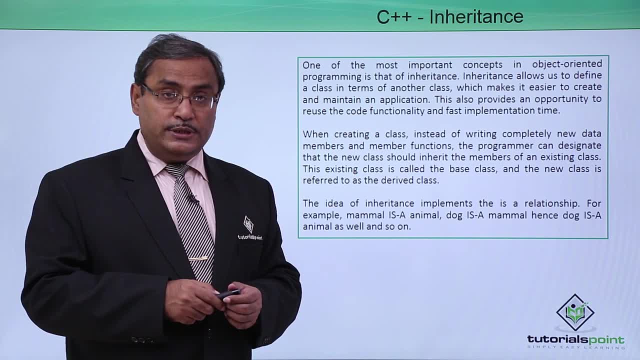 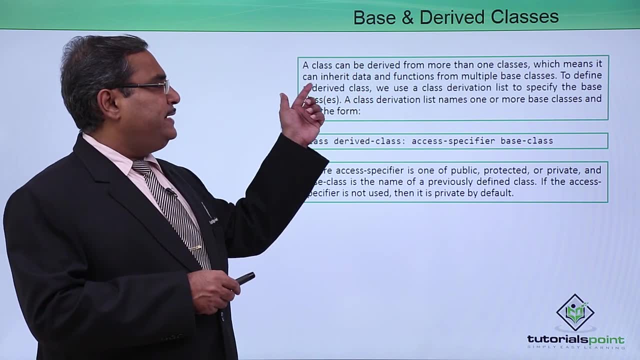 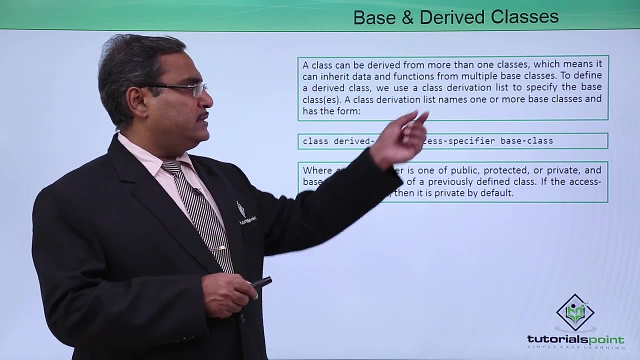 class can be reused in another class using the property inheritance. A class can be derived from more than one classes, which means it can inherit data and functions from multiple base classes. To define a derived class, we use a class derivation list to specify the base classes as well. So here is the syntax. 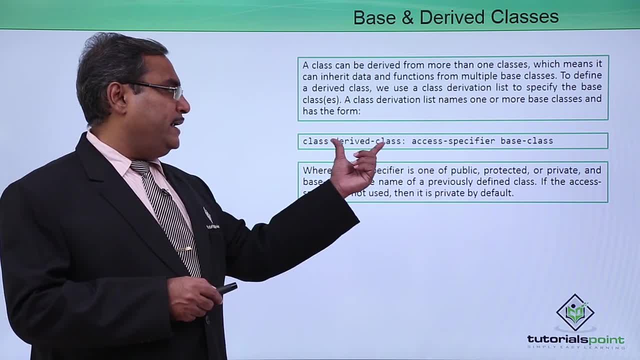 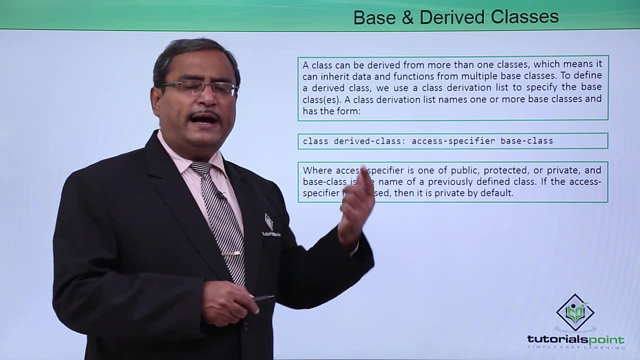 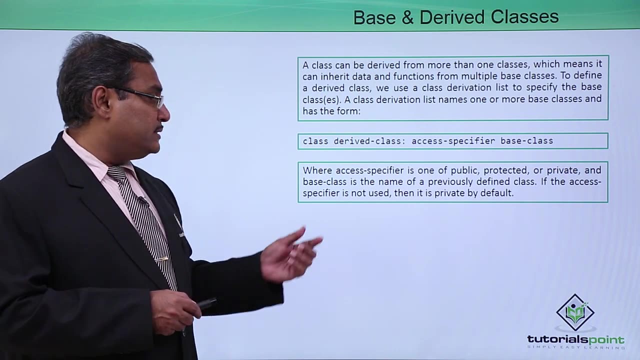 for us. So here this class, then derived class name, then colon will be there, then access specifier base class 1 comma. access specifier base class 2.. In this way we can go on writing: if there are multiple base classes, So where access? 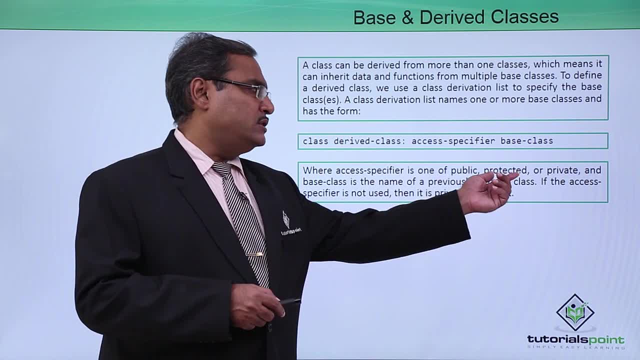 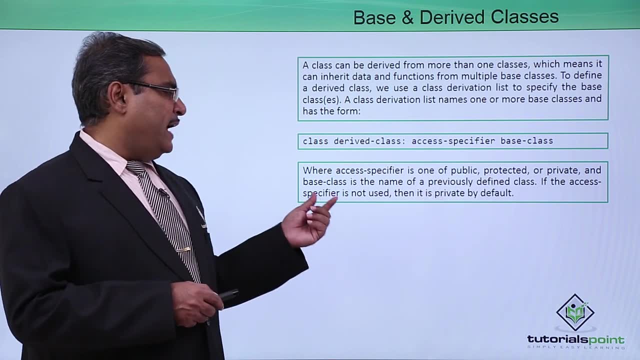 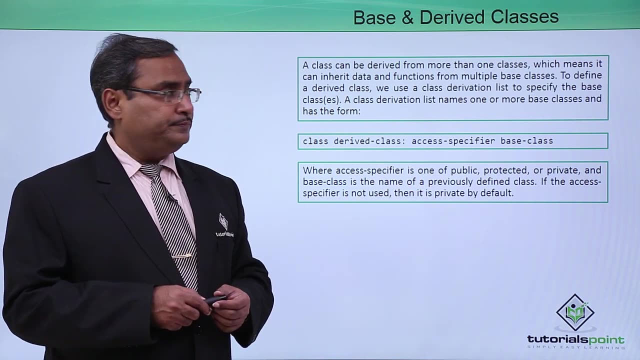 specifier is one of the public or say, protected or private, and the base class is the name of the previously defined class. So if the access specifier is not used, then it is private by default in case of C++. So here one diagram will clear our conception. This is our base class. 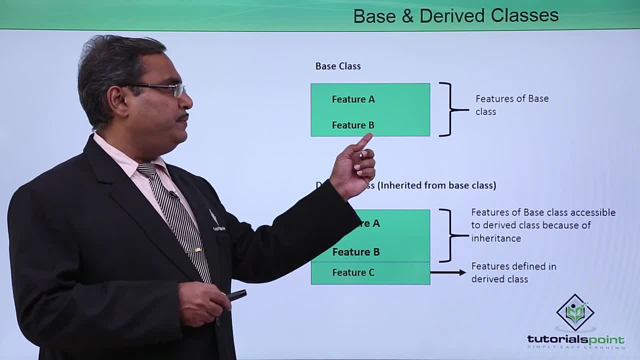 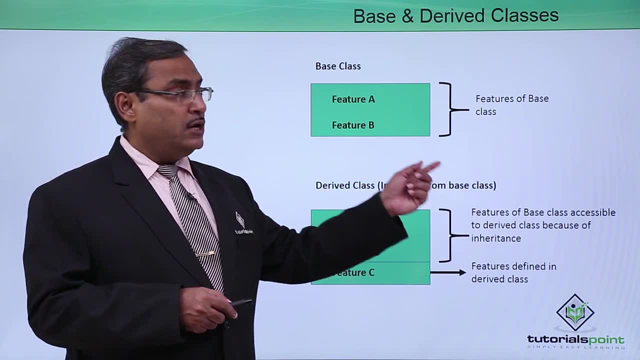 which is having two features. There is a feature A and feature B. So these are the features of the base class and that is one derived class which is inherited from the base class, as well as the following one. Here the base class is an, So these features have got inherited and this base class from the base class, this feature. 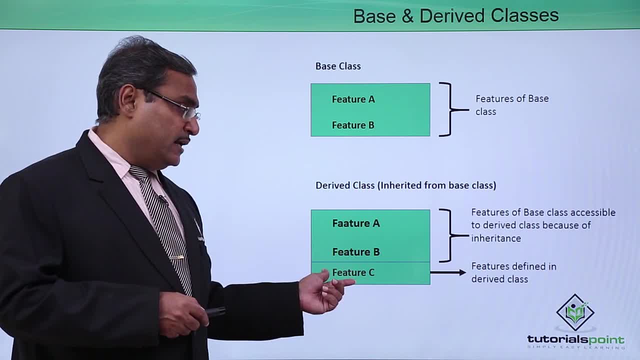 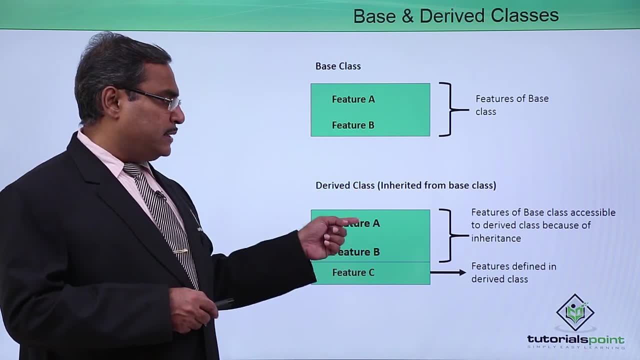 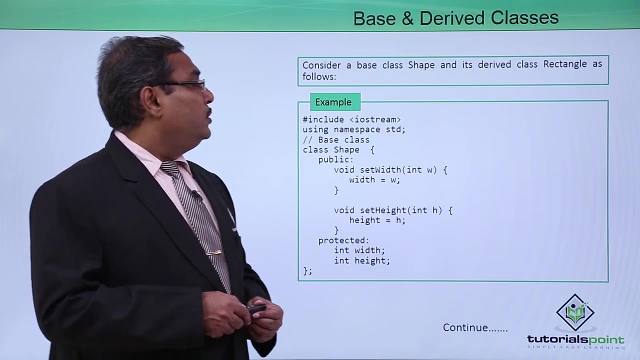 a and feature b. they have come, and this feature c is a new feature which has been introduced in the derived class here. So base class properties are present and derived class can have its extra properties, defined, features defined. So consider a base class shape and it is derived class rectangle as follows: 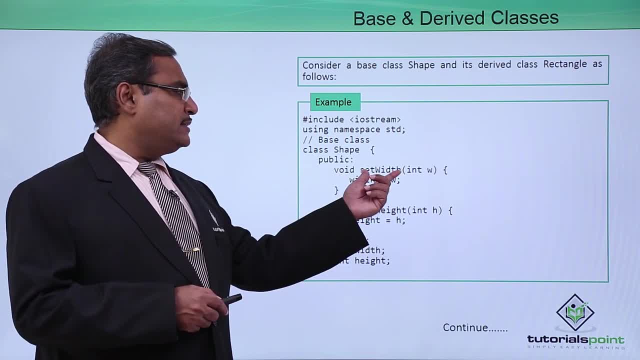 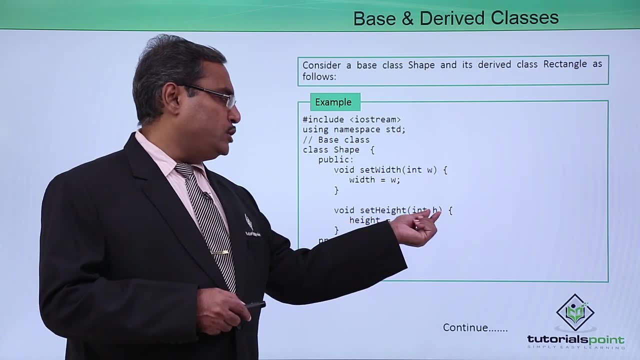 So here we are having one class that is a shape. it is having the set width, where width is equal to w, it will be written in this way. and it is having set height, where h will be passed and that will be kept in height variable. 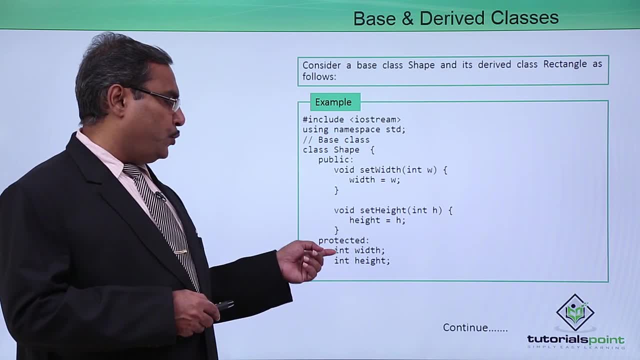 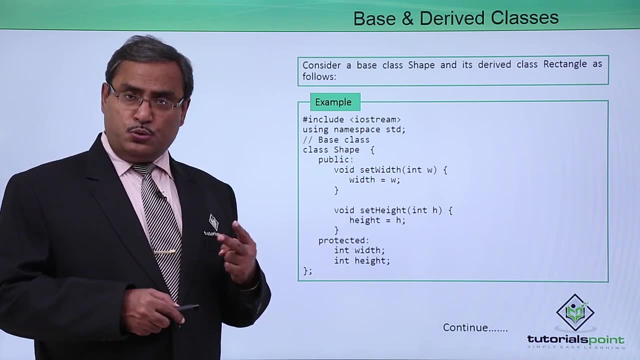 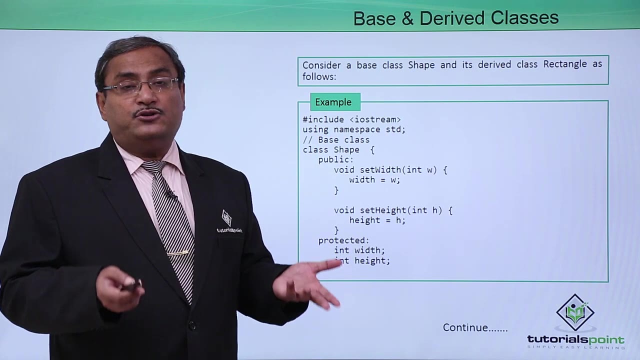 So h will be kept in the height variable and under this protected section we are having this int width and int height. that means the base class shape is having two member variables- width and height, and two member functions set width and set a height. They will actually initialize this width and height member variables. 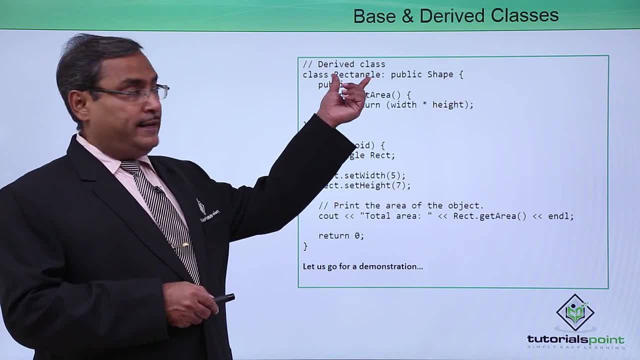 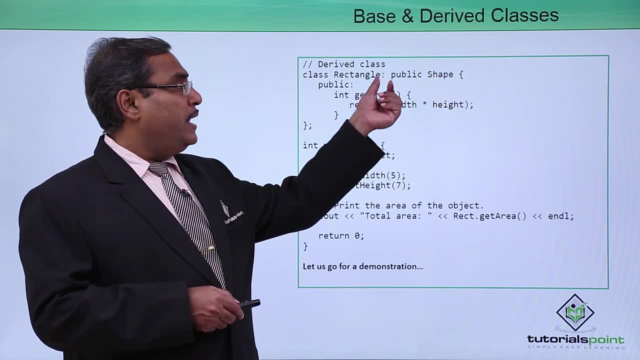 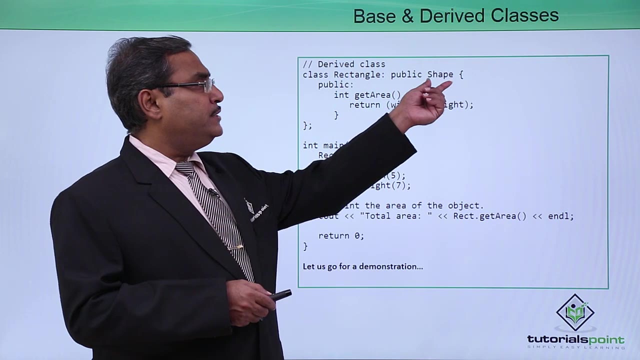 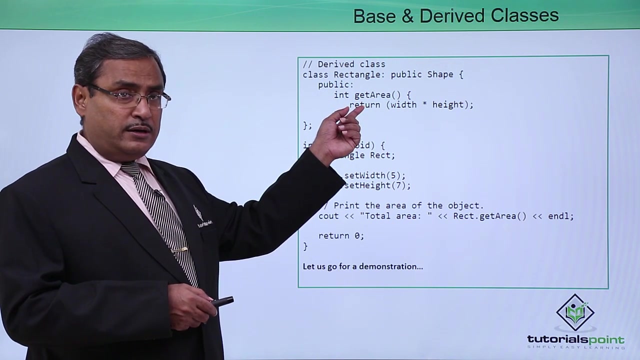 So there is one class known as a rectangle, and here this shape has been called or shape has been inherited, and here this is a scope, is public and colon is according to the syntax. So we have written: class: rectangle, colon, public shape. So here under the public section, in rectangle, we have defined another member function which 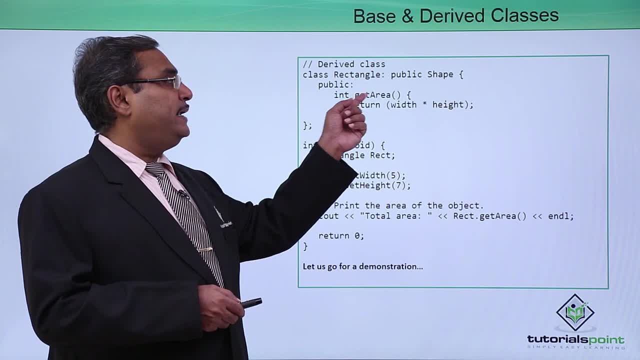 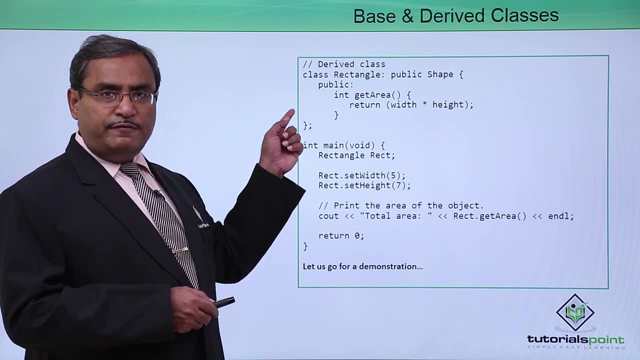 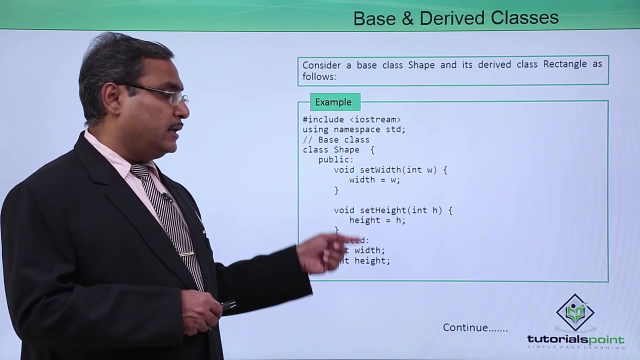 is defined only in the rectangle class is get area, which will multiply width and height. You might be asking me that width and height, they are not defined in this class. then how can I access them? Actually, we have access them because they already defined under the class shape and 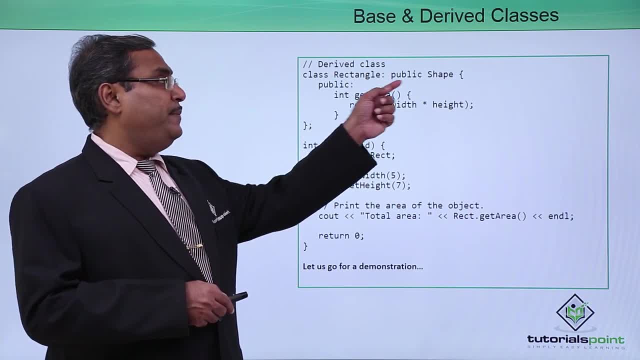 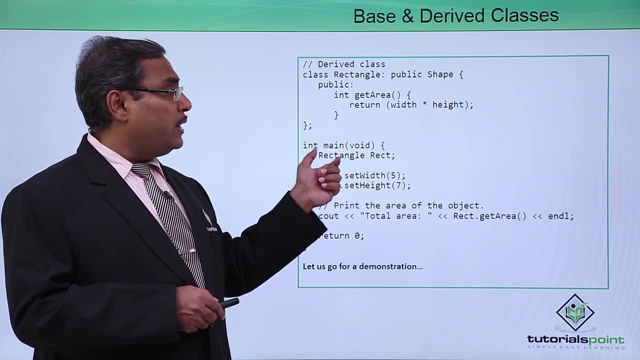 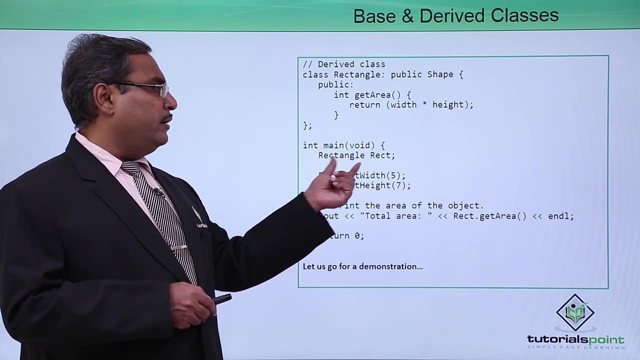 this particular class, rectangle. it has inherited the base class shape, So their corresponding width and height they have got inherited in the rectangle class. So that is why In the get area function I could have access them. So this is my main function. rectangle class is having the object rect and then rect dot. 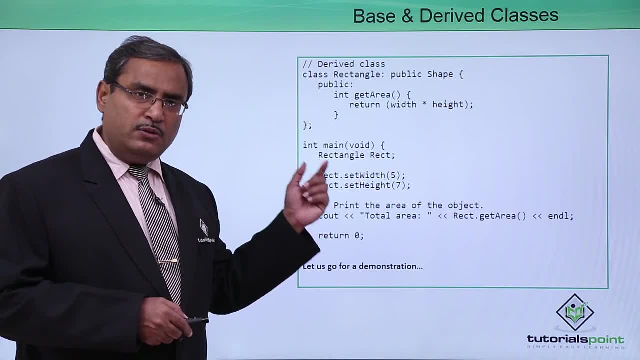 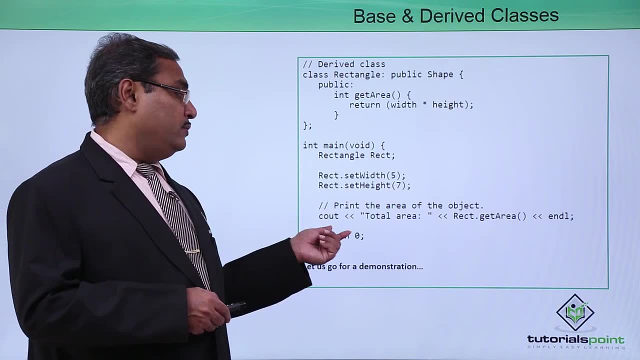 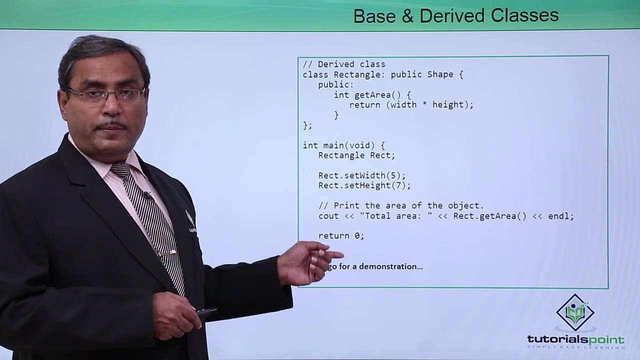 set width: 5 will be assigned to the variable width, and rect dot set height: 7 will be assigned to the required height in the height variable. and then we are calculating the area using the function get area and that has got printed and then the program has got terminated. 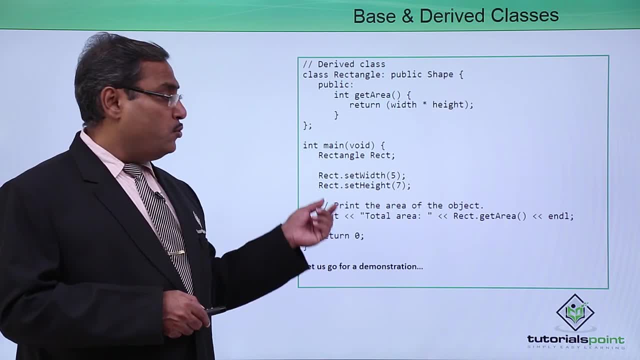 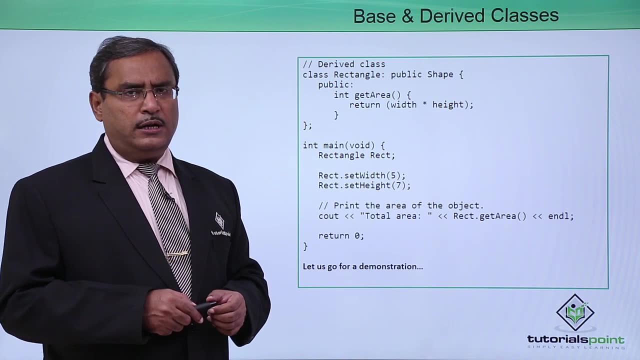 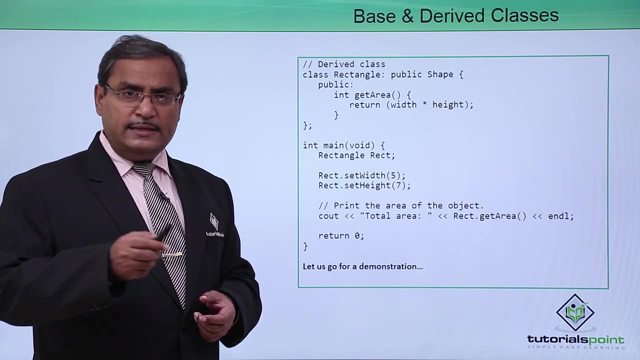 So here, to access the Required members, we are using this dot operator. So for the better understanding of the code, let me show you one practical demonstration where this code will be compiled and executed and outputs will be explained once again to you. So here is the demonstration for you. 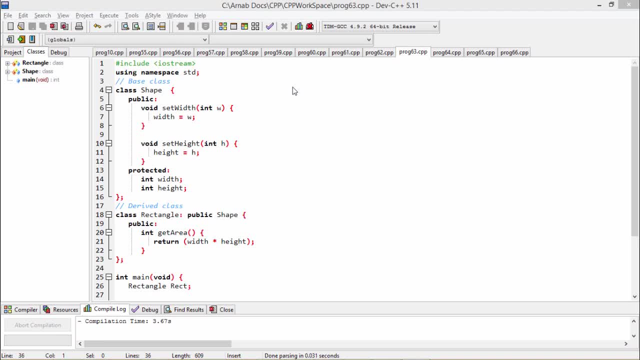 Let us explain this program. here we are defining one class, known as the base class, and this class is having the name shape Under the public section. Under the public section, we have defined set width, one member function, set height, another member function, and two variables under the protected section, under the protected scope. 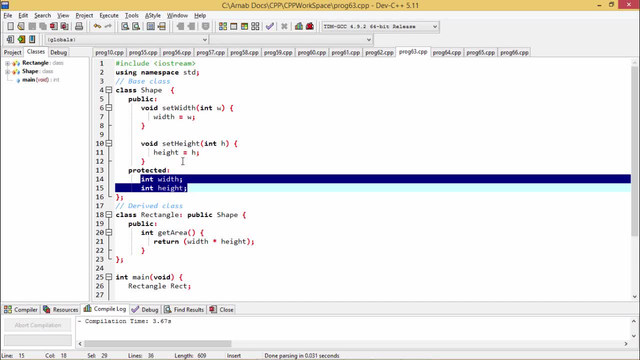 So here we are having int width, int height. this set width and set height. they are taking the respective values as input argument and those values are getting assigned to the respective member variables. And that is the purpose of this: to set our functions, set width and set height. 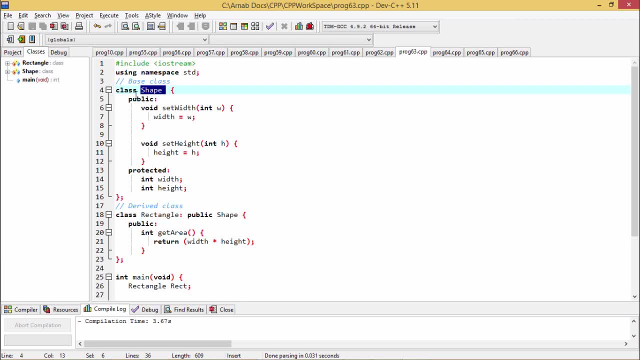 So name of the class is the is shape and this is a base class because this particular shape has got inherited in the class rectangle under the public scope. So shape is the base class, rectangle is the direct class and this rectangle is inheriting properties from shape. 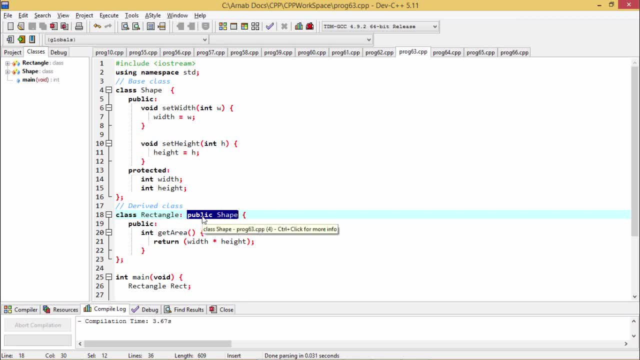 And here we have defined the base class. So here we have defined the base class, this public scope here. so, as a result of that, all the public members of this shape will be coming to the public section of this rectangle and all the protected member variables will be coming to the 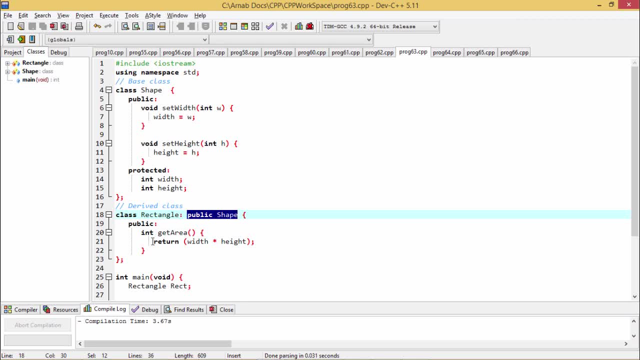 protected section of this rectangle class. so here we have defined one extra member function under the scope, under the section public, so return, which is returning the product of this width and height as output argument. so that's why int is the product data type. so now in the main function we have defined one object under the class rectangle, the name of the. 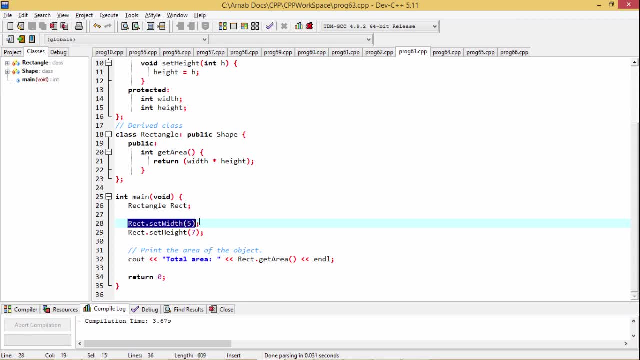 object is rect, so we are calling this setter functions, as these setter functions got inherited in the public section, so object name dot operator using we can access them as well. five has been passed as input argument to this set with, and this five will be assigned to w and that will be. 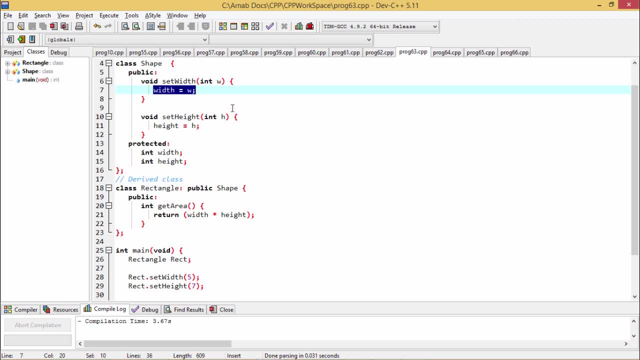 assigned to the member variable that is our width in the class. so in this way, the set height is taking this 7 as input argument. so this 7 is getting assigned to h and then it is getting assigned to the height member variable. so now, after getting them, we are calling this rect dot gate area. you can find that this gate area. 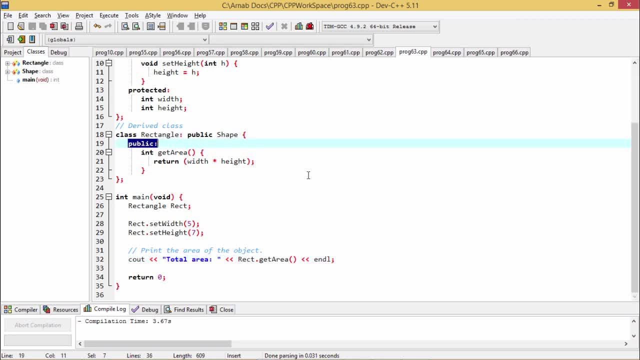 is also under the scope public. so as a result of that, it is accessible from the outside of the class through object name dot operator. so in this way, the total area is getting printed by multiplying this width and height. so for the better understanding, let us execute our problem. 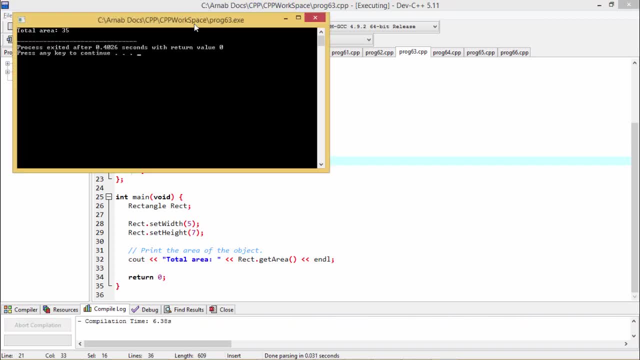 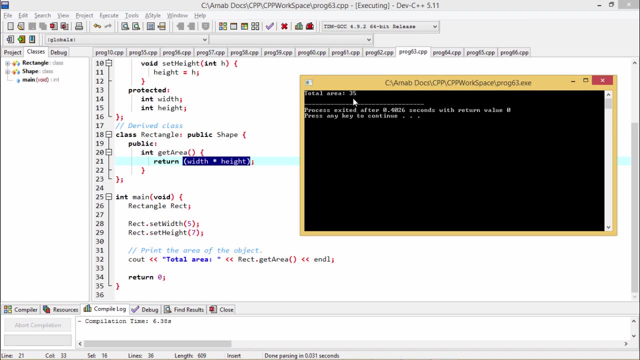 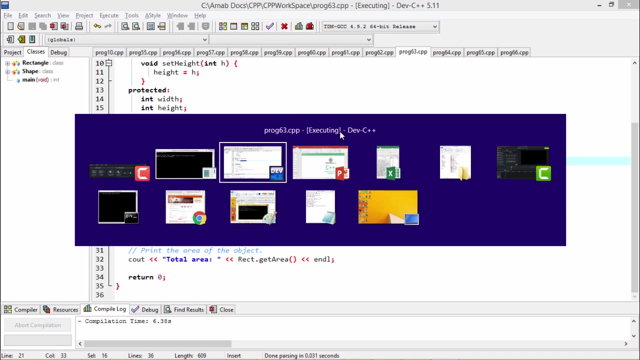 so that's why you have clicked on compile and run option. and we know that if we keep the value five and seven, then the respective area after multiplication, after multiplication, will be obtained as 35.. let me execute the same using our gnu c plus plus environment. okay, so here we are, having this particular 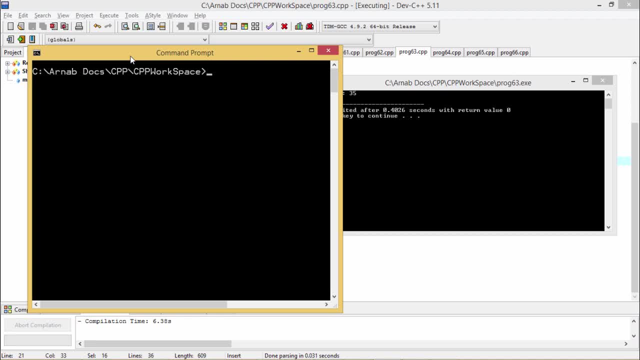 options. so now here the program name is proc 63, so going for g plus plus 63 dot, cpp minus o, a, dot ex will be the output file name. i'm going for the compilation. compilation has got completed successfully. now i'm executing. i'm getting the same output as i got. 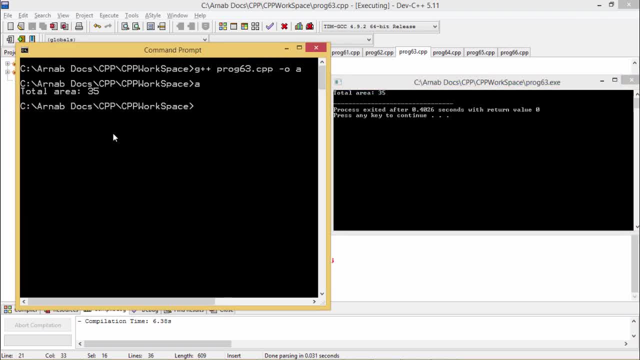 in case of depth c plus plus execution that is practical in this way. this program we have explained line by line and also we have shown you the output after running it in the depth c++ id and also running it using g nu c plus plus compiler. thanks for watching this video.